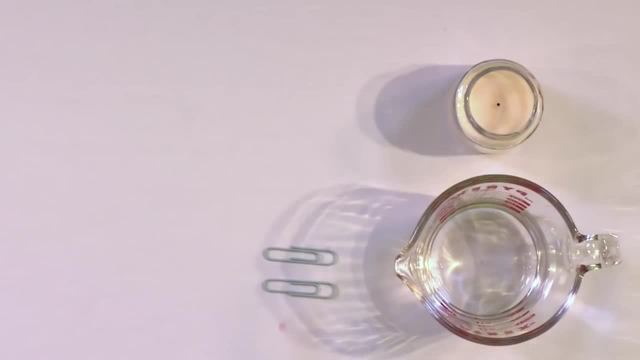 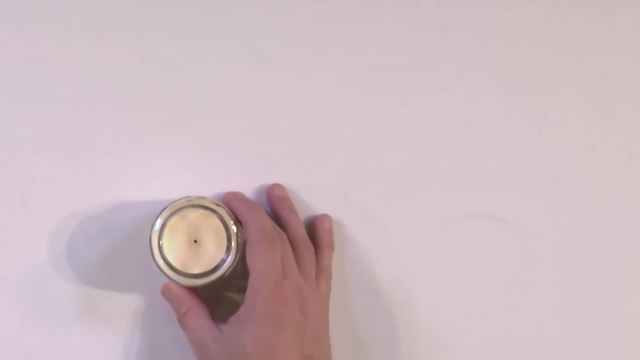 balloons closed, All right. so what we'll do is go ahead and get set up here. We'll put the water to the side, put the balloons to the side, We'll put the candle front and center and we will light the candle. So let me go ahead and do that first, All right? 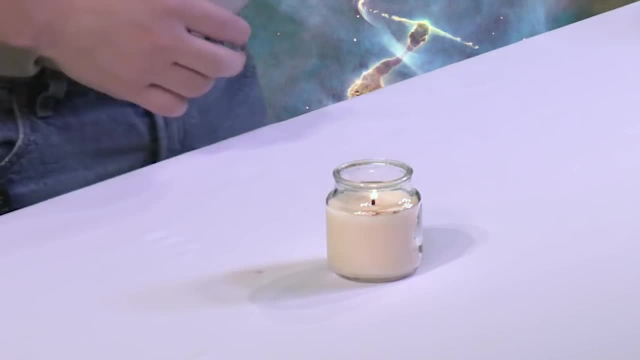 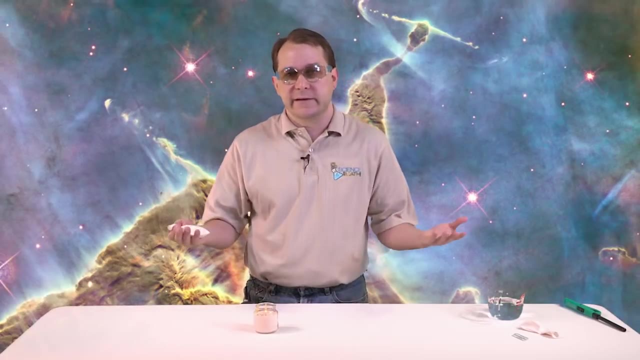 so it just takes a second to go ahead and light the candle. The candle's lit And the next thing we're going to do is we'll show you what happens to a regular old balloon whenever you put it in here. What do you think is going to happen? Well, if I blow this up, 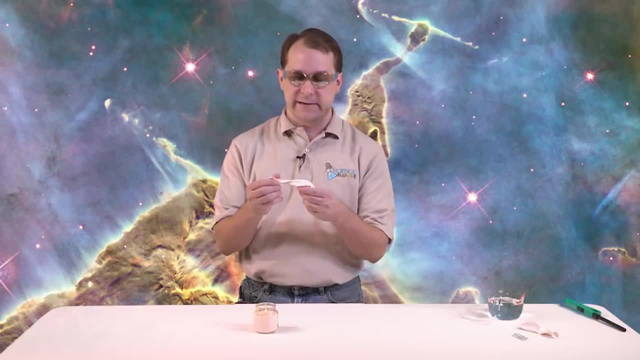 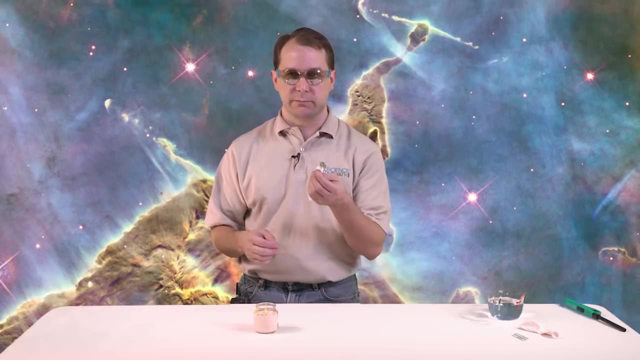 and I put it on top of that candle flame. the hot air is going to go, It's going to hit that rubber, It's going to melt it a little hole and then pop. the balloon goes, pop. So let's go and check that out. I'm going to go ahead and blow this up. 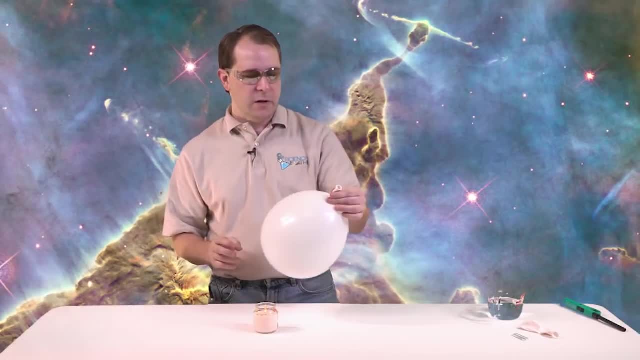 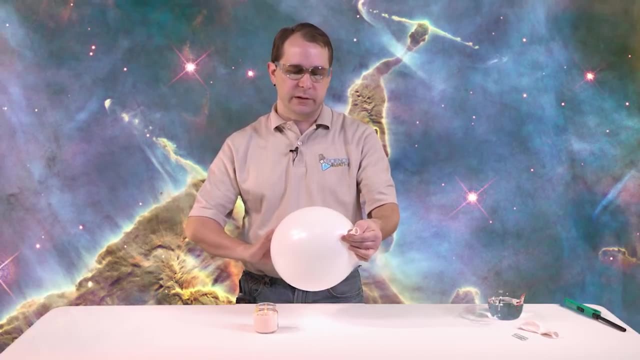 All right, so there we go. So I'm going to blow it up. Now you can tie it if you're really good at tying balloons. Tying balloons can be difficult, So if you want, you can. just once you get it blown up, you can just twist it a few times like this. So I've got a nice. 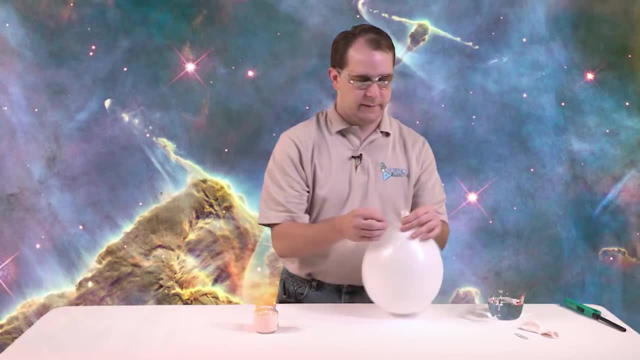 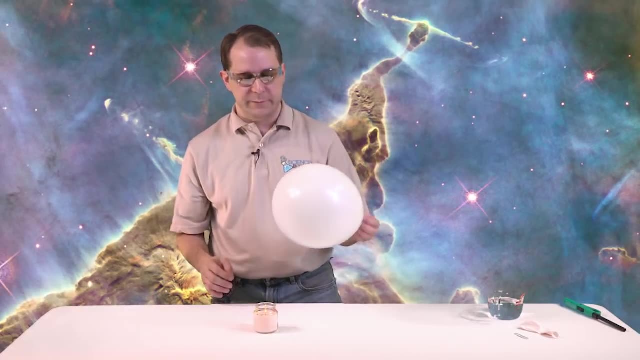 little twist at the end And then grab one of my paper clips there and just put it right on top of that guy And if you've done it nicely, you should be able to hold the end of it and just kind of keep it closed. 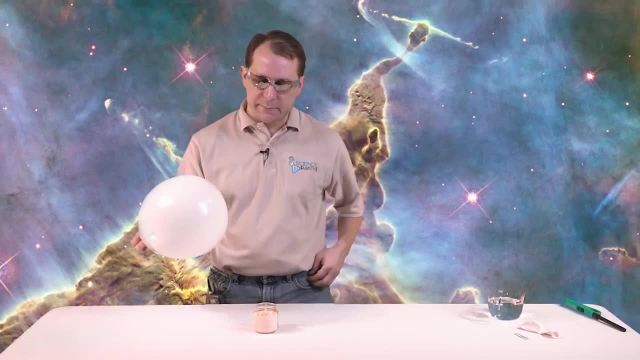 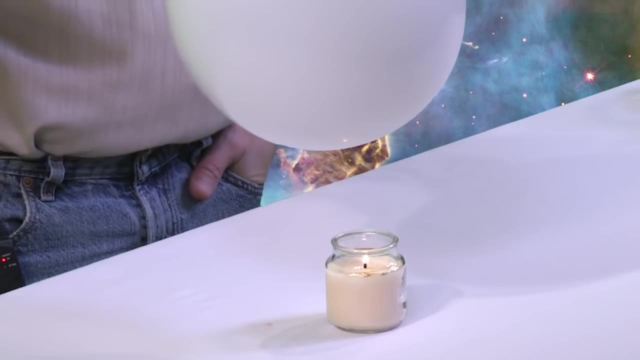 All right. so what do you think is going to happen If I put this guy right on top of this candle flame? it should pop, right. So let's check that out. So we'll put it there. Let's see how close we can get before it goes. pop A little bit down and there it goes. 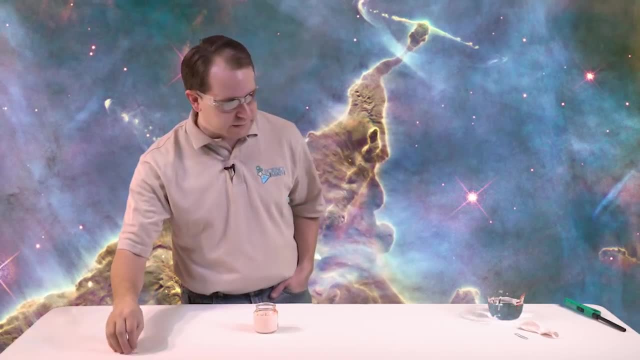 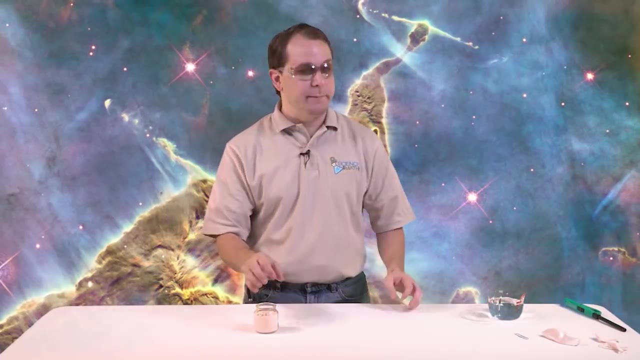 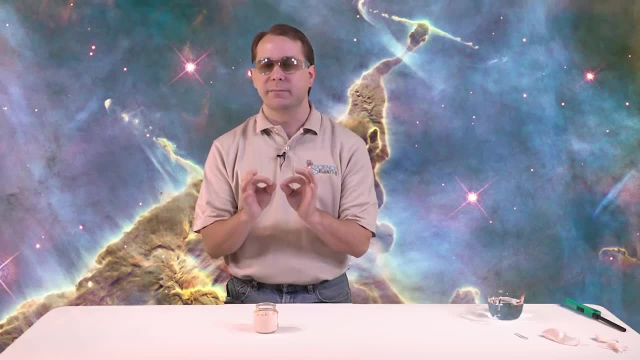 pop, So it's going to pop, So it's going to pop, So it's going to pop. So the candle flame went directly to the rubber, made a tiny small hole in that rubber because it melted it, and then, as soon as it made a small tiny hole, the whole thing just kind of pops. 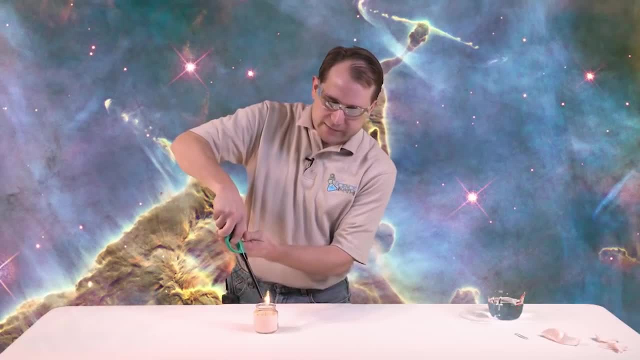 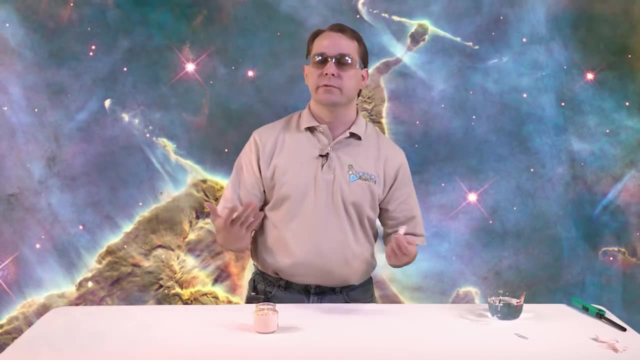 Right. So that's what we kind of expect. Let's go ahead and relight the candle. It looks like our balloon actually put out our candle flame. Now, the second time we do it. that's why we have two balloons. first time we show you what it looks like regular. Now I'm going. 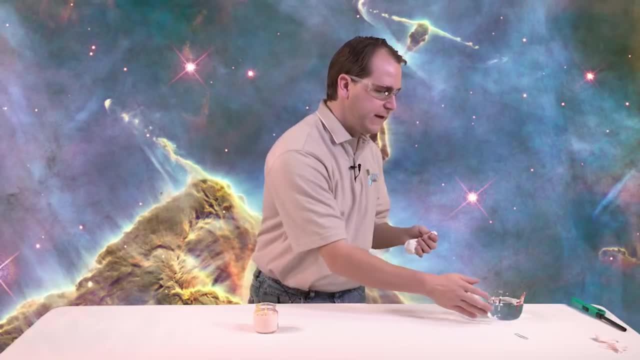 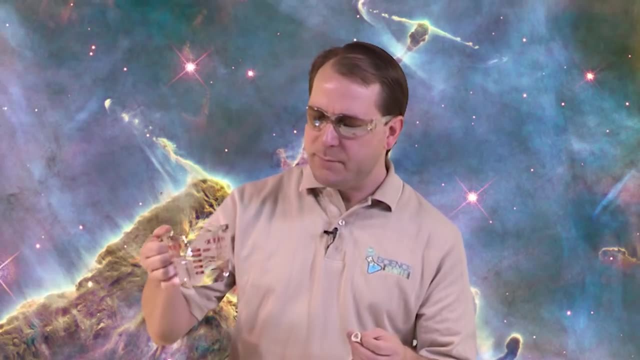 to do the same thing again. but now what we're going to do is put a little bit of water in our balloon. We're not going to fill this balloon with water. We're going to put a little bit of water in it, maybe even less than half a cup of water. 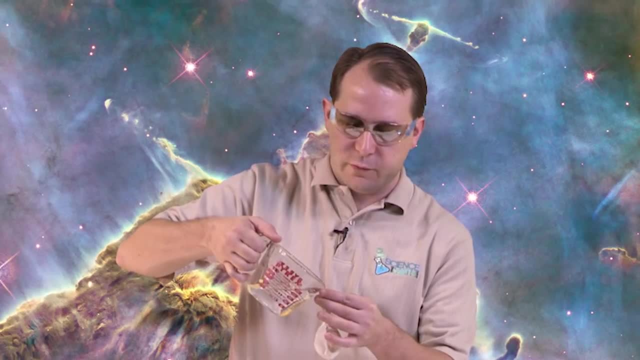 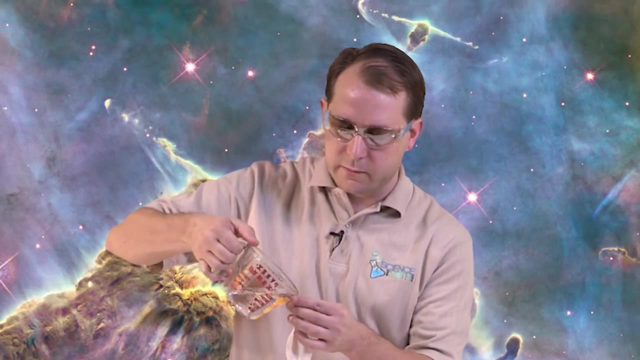 So what I'm going to do is just pour a little bit of water into the bottom. So now I have a little bit of water, I'm going to put a little bit more. I would guess, well, maybe that's like probably four or five tablespoons of water. 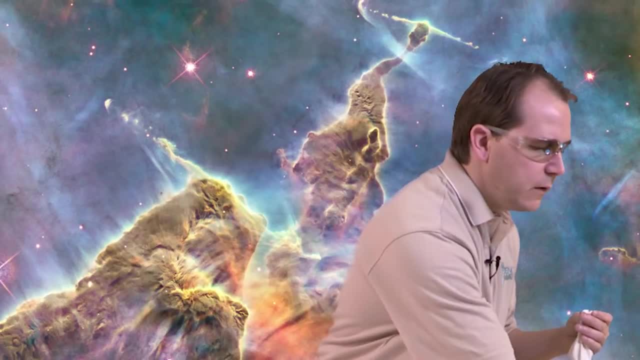 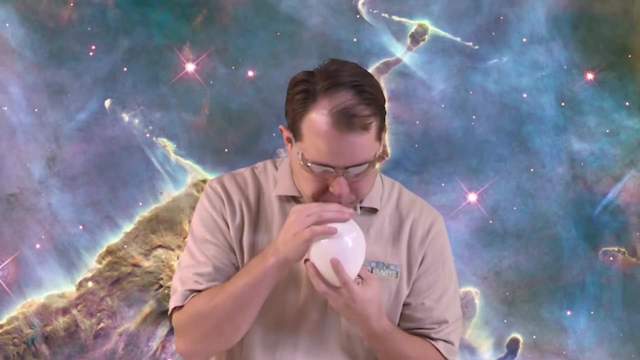 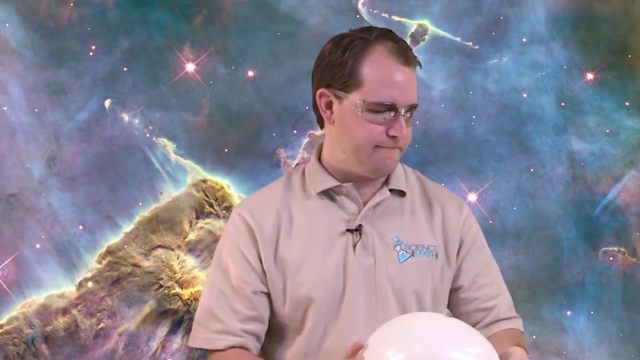 really is all. it is Okay. So we're not filling up the water, We're just putting a little bit of water in the bottom of the balloon. Now I'm going to go ahead and blow it up again. Now we're going to go ahead and twist this guy up. 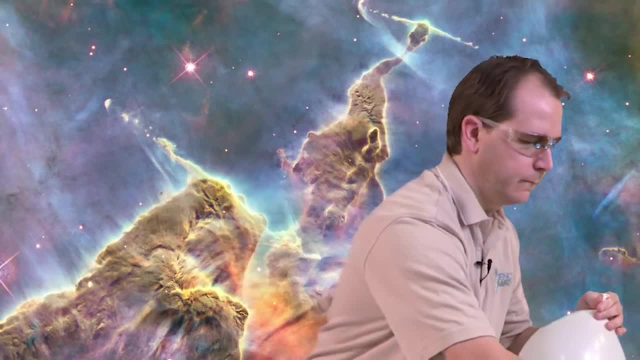 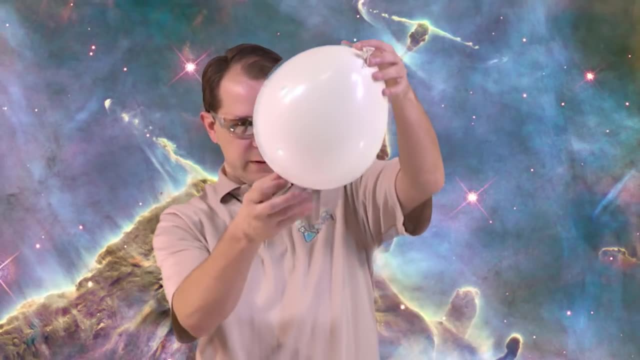 just like we did the last time- nothing different- And put that paper clip on there to hold it there. Now what we have is a balloon and if we've done it all correctly, we should have water sloshing around the bottom of this balloon. 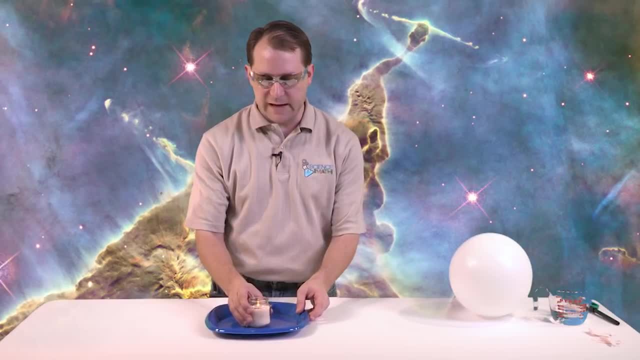 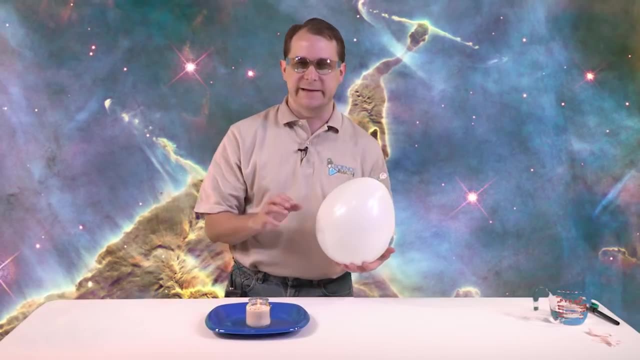 Now, before we do the second part, where we put the balloon on top, I'm going to put my candle on a little plate. The balloon shouldn't pop, but just in case it does, we want to have a little plate there to try to catch at least some of the water. 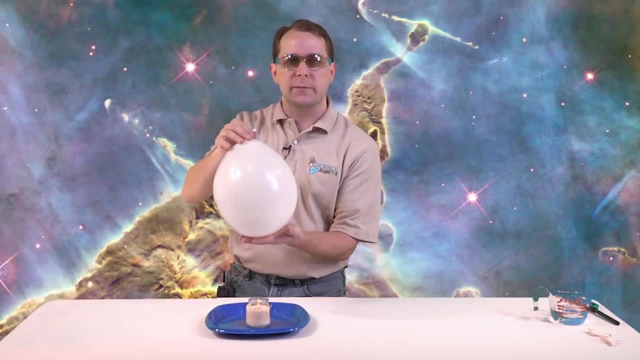 So what you want to do is you want to put- you know you have the water in the bottom of the balloon and you want to put it right on top, the same place we had before, And let's go ahead and give it a good count to five. 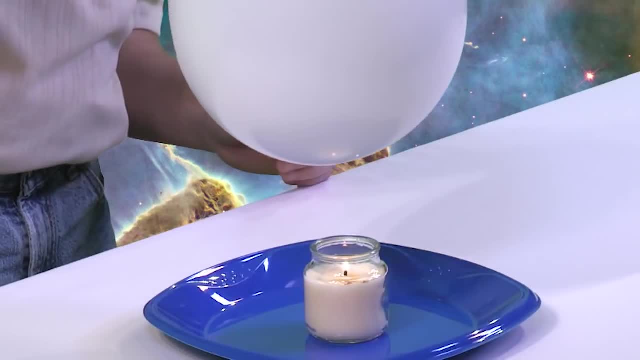 and see if we can get this balloon to last. So let's go down One, Two, Three, Four, Five. Now, if you put your hand to the bottom, it does feel a little bit warm, but it's not super hot. 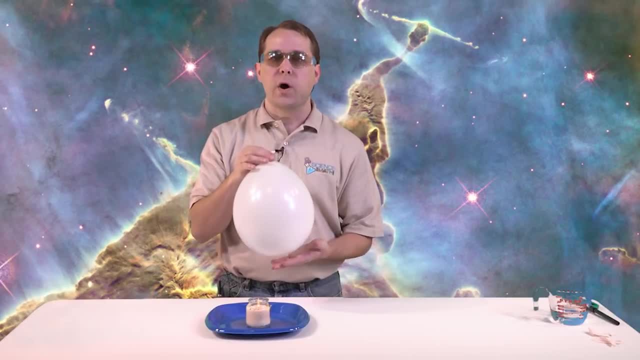 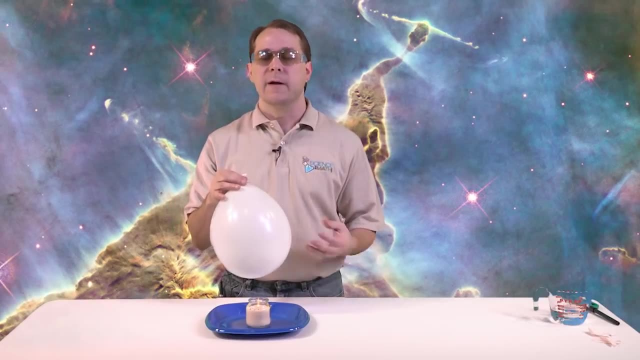 Why do you think that is? It's because you have water inside of it. So what's happening is the heat from the candle is going into the rubber, and normally it would pop that rubber, but since there's water in it, water is a great absorber of heat, so to speak. 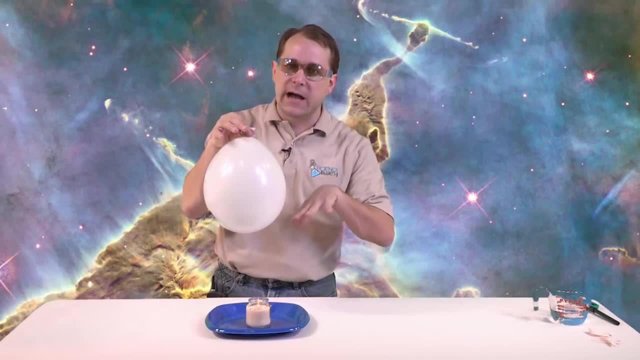 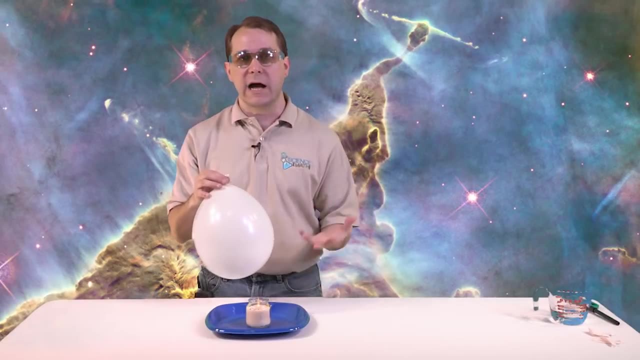 So what happens is you put the heat into the rubber. the water is sitting right behind the rubber on the other side. It's absorbing all the heat, So it's kind of pulling it in. It loves to take in that heat, and water can absorb a lot of heat by itself. 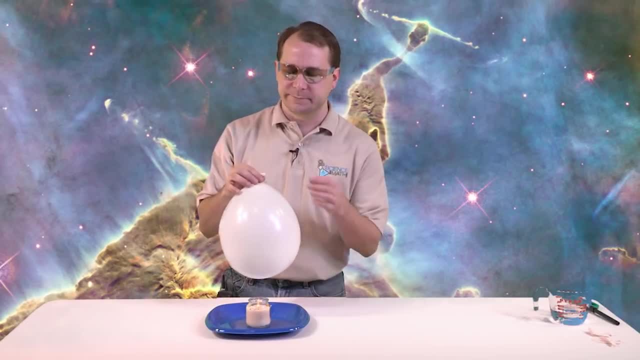 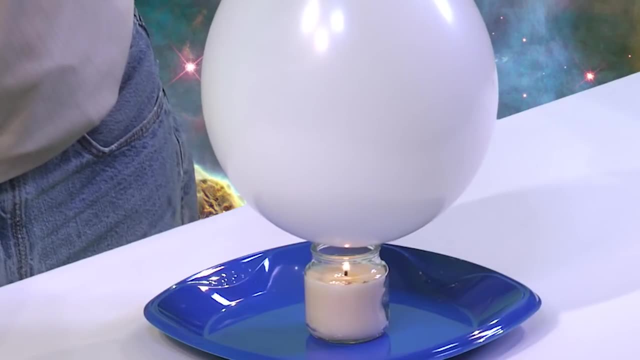 So it kind of takes the heat away from the rubber and that kind of prevents it from popping. So let's go ahead and try it one more time and put it even closer. We'll go even a little bit lower, Right on top. 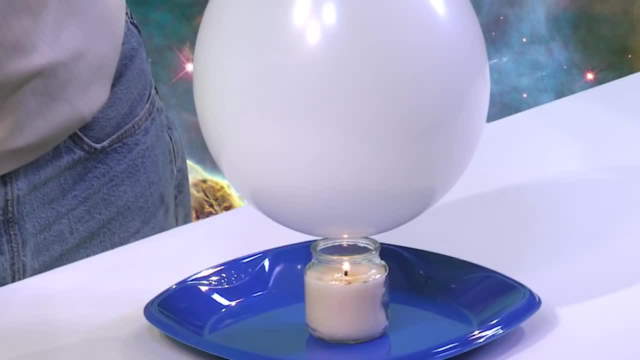 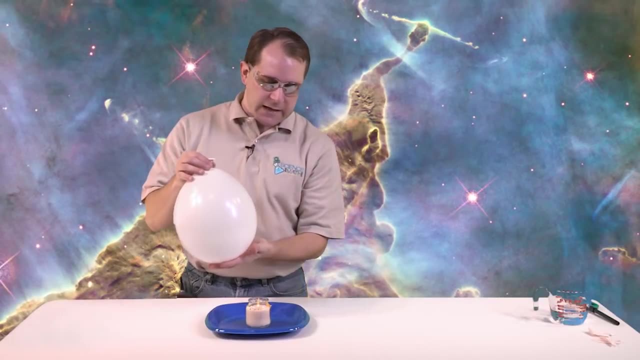 And you can see that definitely it would have popped by now. And put your hand on the bottom, Not too warm. And so, for our grand finale, what we'll do is we'll put the balloon directly on top of the glass and see if, by putting it right on top of the glass, 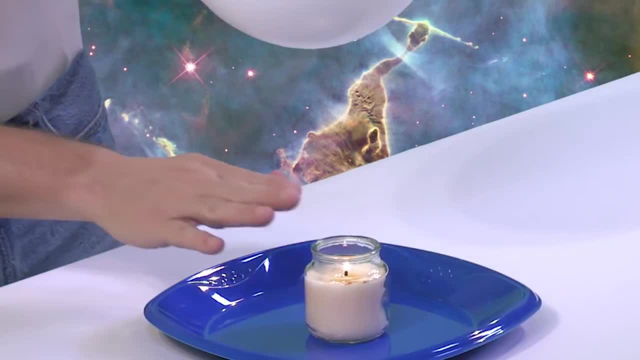 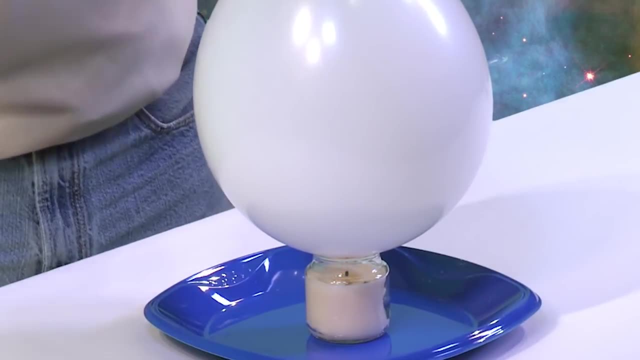 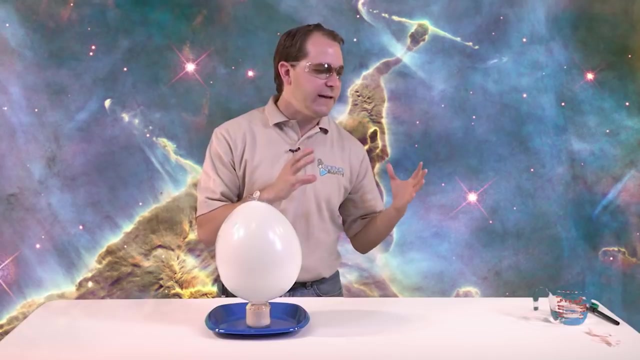 we can actually smother the candle. So that would be sort of the grand finale, All right, And so we'll just put it right down there And the candle is out. So that is a good experiment in, basically, heat conduction. We did the empty balloon. 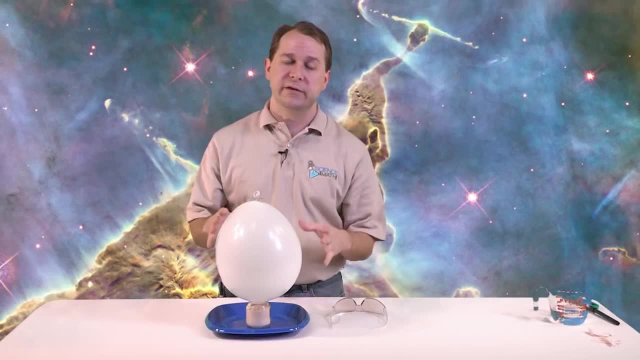 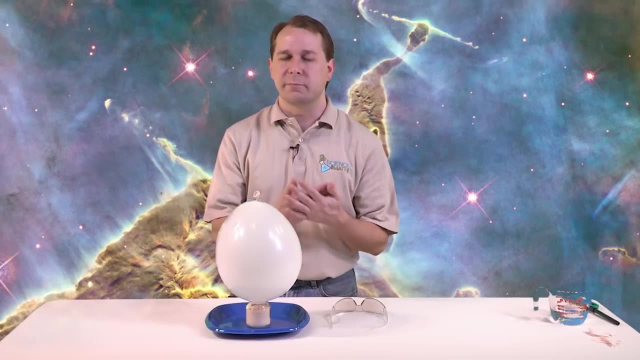 and that showed us that if you have an empty balloon, you put it on top of a candle flame, it's definitely going to pop. And the reason it pops is because the hot air that's coming off of the candle basically melts a small 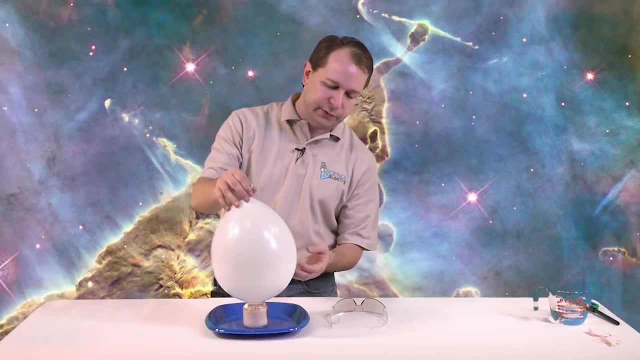 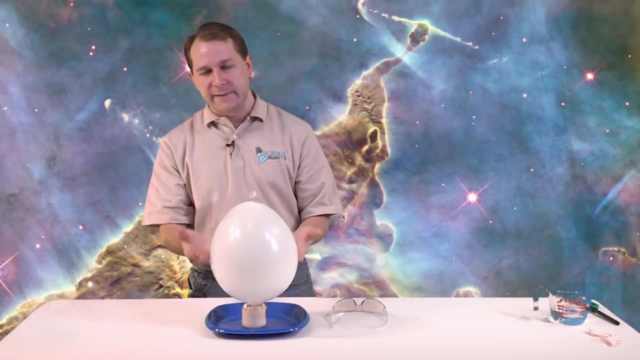 tiny hole in the balloon and then it pops, And really the other balloon I mean it was very, very, very close to the actual candle, but it wasn't even touching the candle before it popped. In this case, what we did is we take the full balloon. 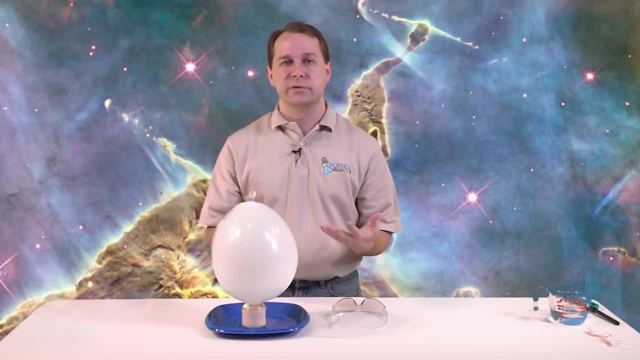 and we put some water in it and then the heat goes from the candle into the balloon and then it goes into the water that's sitting right on the other side of the balloon. That water is pulling that heat, conducting that heat away from the rubber. 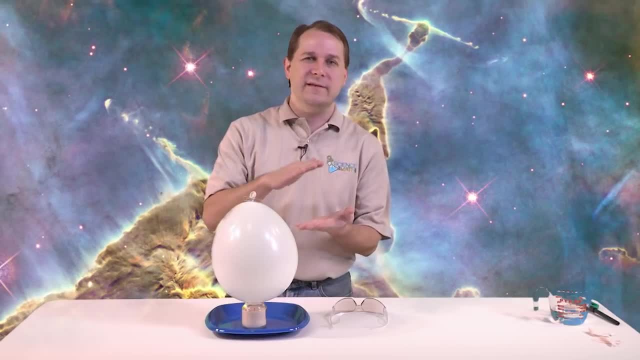 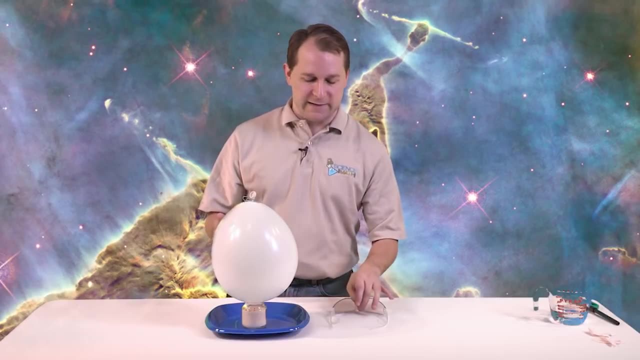 So the bottom line is the rubber is not able to get that hot because as soon as it does get a little bit hot, the water sucks that heat away. So that's what causes the rubber not to melt and not to pop. And you know, we have a bonus science experiment here. 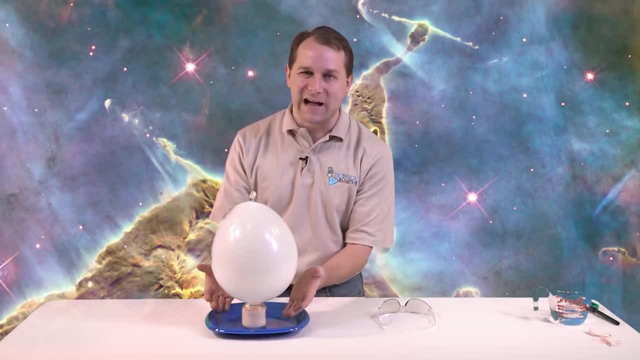 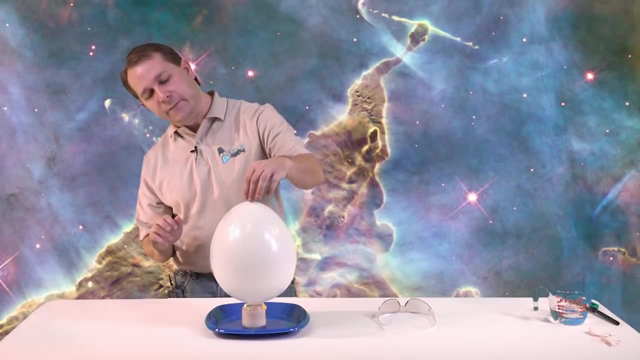 What we did is we kind of put. we put the balloon directly on top of the candle, right to smother it, just to show you how close we could get to it. And look what happens now If we lift this balloon, try to lift it off. 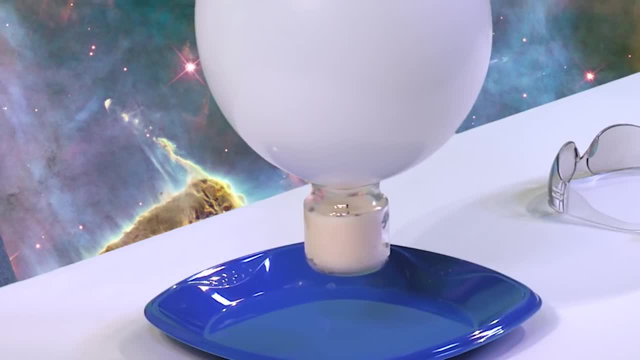 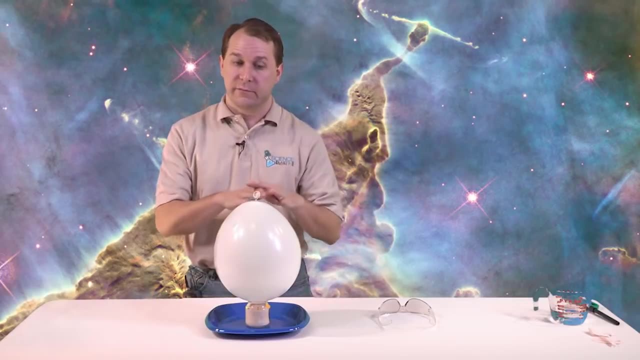 we can actually lift the candle. Now why do you think that's the case? It's sort of a bonus science experiment. What happens is the air that's directly around that candle, down where the flame is, is very, very hot, right.